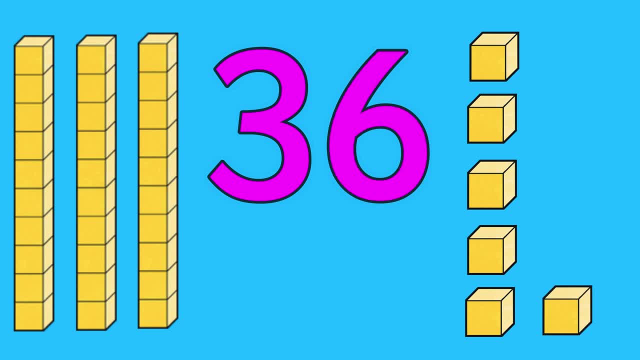 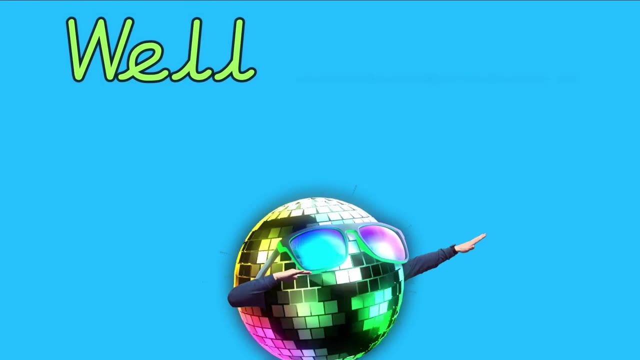 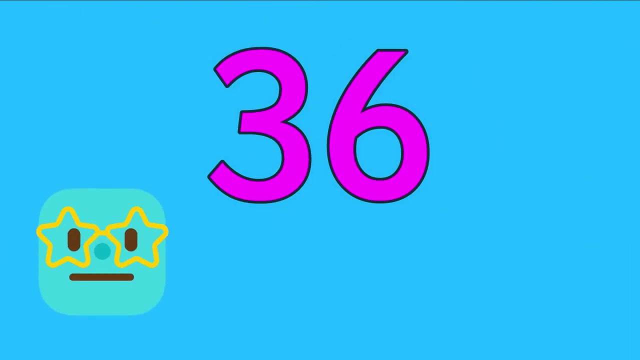 now let's count them all together: 10, 20, 30, 31, 32, 33, 34, 35, 36. well done if you joined in with the counting. now that we know what 36 looks like, let's have a go at making it. 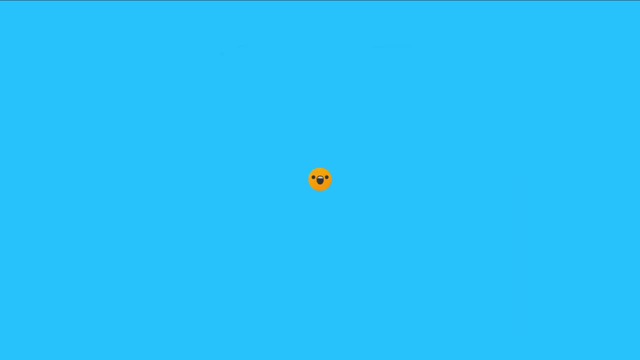 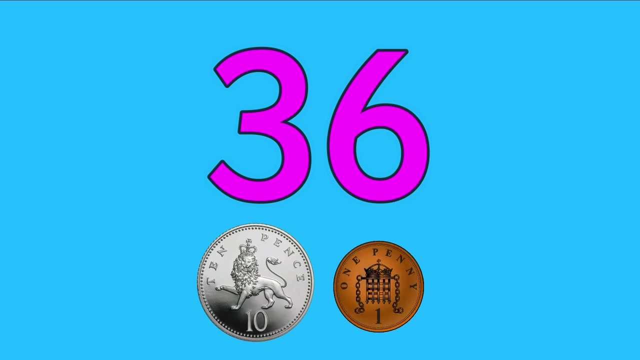 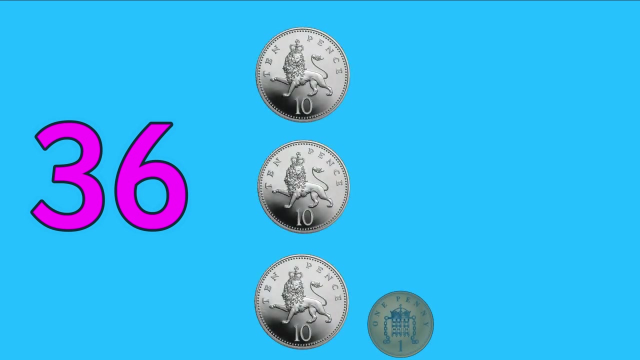 in as many ways as possible. did you know that there are tens and ones all around us, like with money? let's make 36 with 10ps and one piece. join in with me. 10, 20, 30, 31, 32, 33, 34, 35. 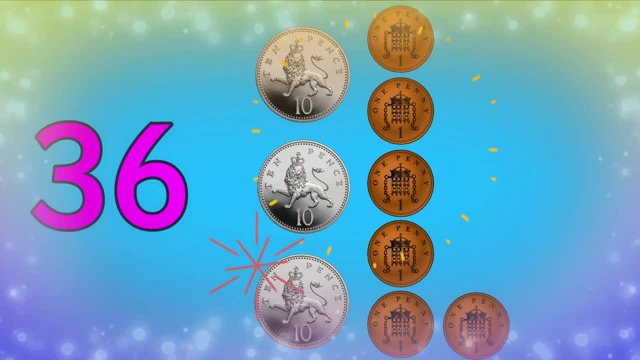 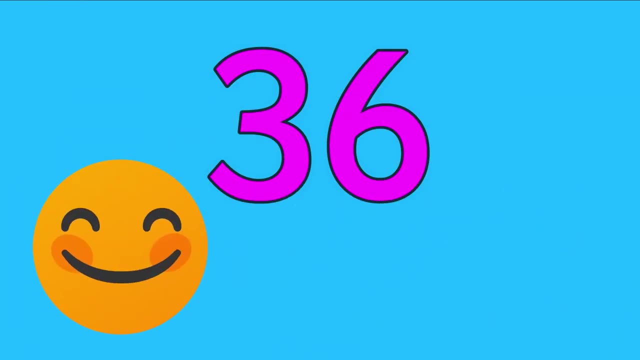 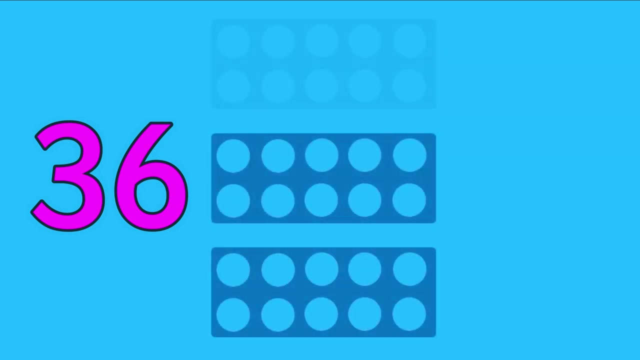 36. hey, we made 36 using tens and ones with money. now let's try making 36 using Numicon. we will use the ten pieces and the one pieces. join in with me: 10, 20, 30, 31, 32, 33, 34, 35, 36. 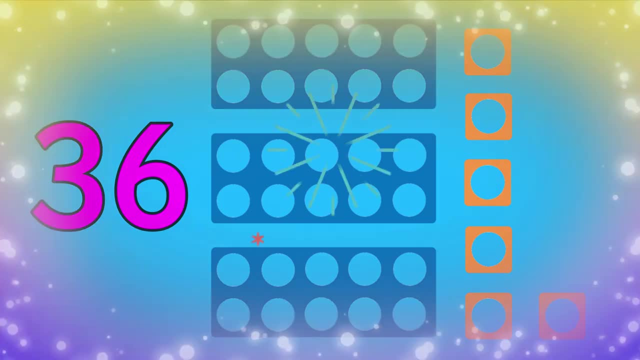 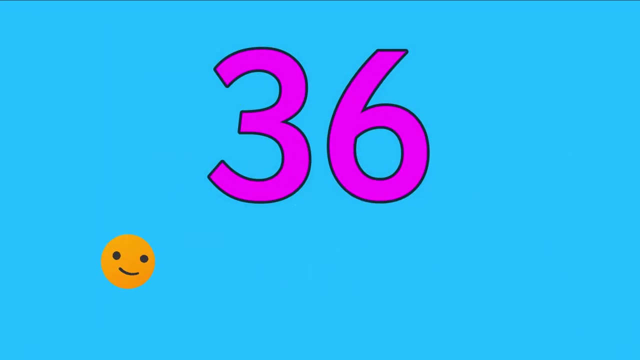 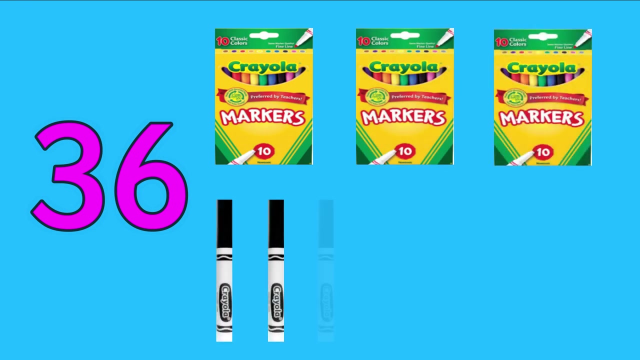 We made 36 using Numicon: 10s and 1s. Now let's make 36 using pens. We will use some 10 packs of pens for the 10s and some single pens for the 1s. Join in with me. 10,, 20,, 30,, 31,, 32,, 33,, 34,, 35,, 36,, yay. 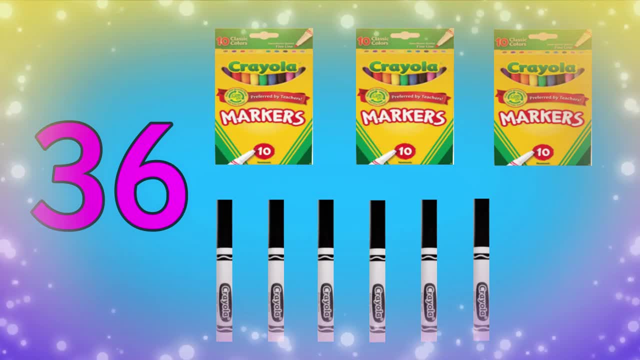 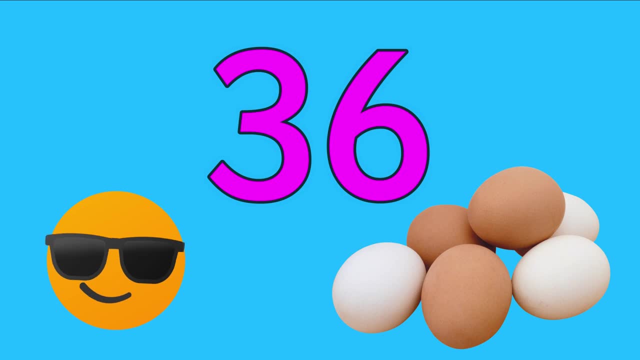 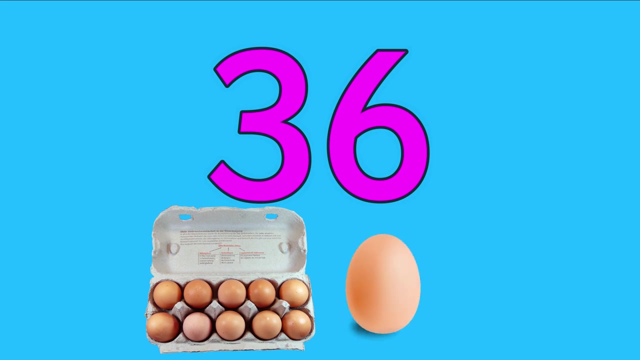 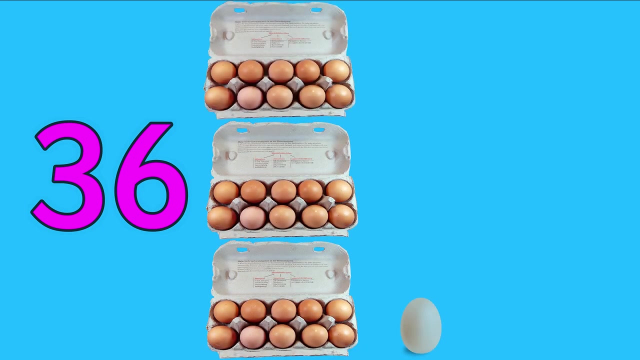 We made 36 using 10s and 1s with pens. Now let's make 36 using eggs. We will use some 10 packs of eggs for the 10s and some single pens for the 1s. Join in with me. 10,, 20,, 30,, 31,, 32,, 33,, 34,, 35,, 36,, yay.